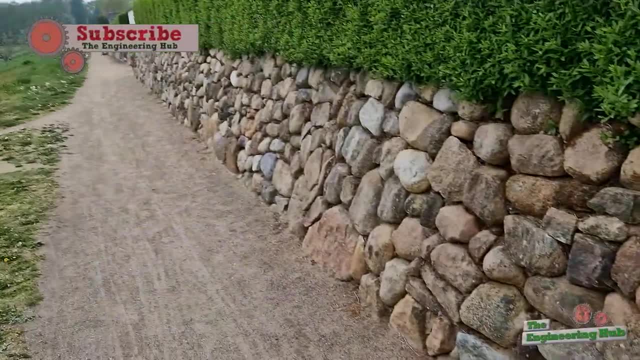 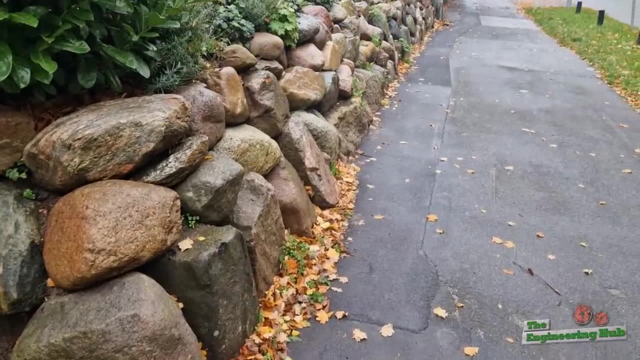 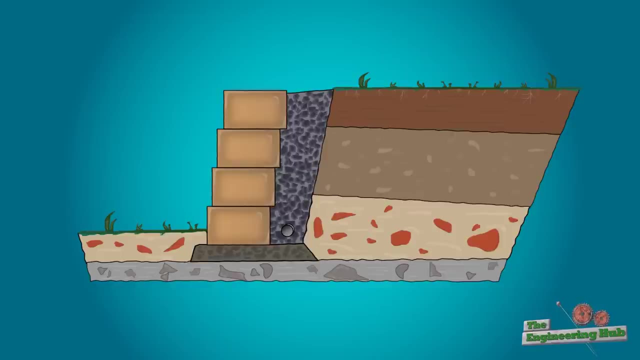 the upcoming videos on foundations and slope stability. If you are enjoying these videos, consider writing a comment or clicking the like button. this helps us greatly. Now onto the design considerations. The design of retaining walls can be approached from two directions: either increase the resistance of the wall or decrease the earth pressure. 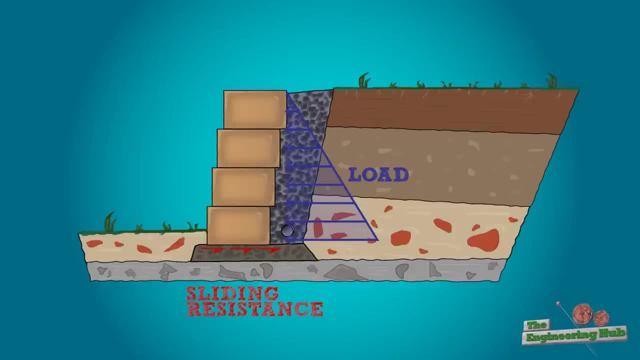 Let us first look at the resistance side, since it is fairly simple. Gravity walls use their own weight to retain the soil mass. The weight of the wall induces a frictional force at the bottom of the wall that prevents sliding, Embedding the wall into the ground. 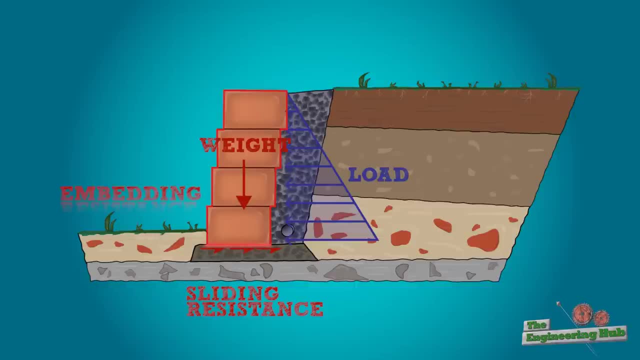 can add an additional component of resistance which helps greatly. Extending the base of the wall into the backfill helps activate the soil mass as part of the wall and increases the base friction and resistance to overturning. But this usually requires more excavation and could increase the cost significantly. 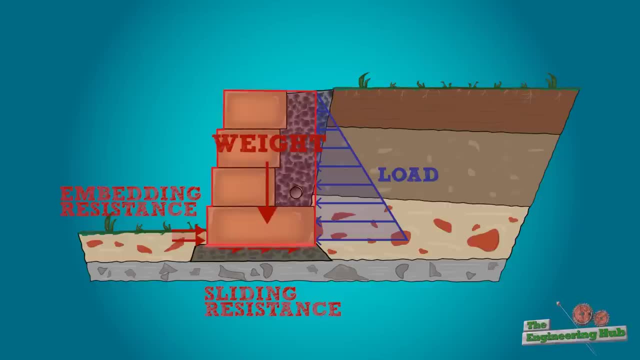 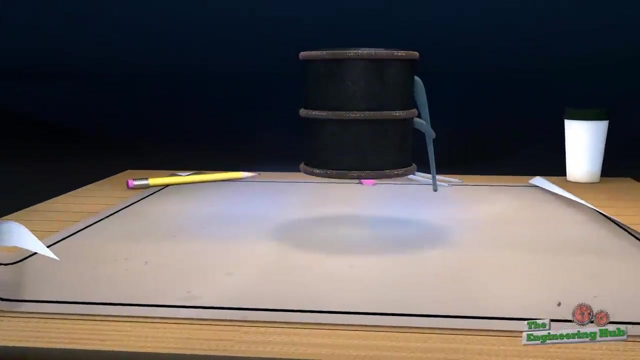 Increasing the size and therefore the mass of the wall could do the job, but this is also a costly solution. In practice, engineers tend to pay more attention to the soil behind the wall and reduce its effects. Soils act similar to water in the sense that they exert pressure on its surroundings. 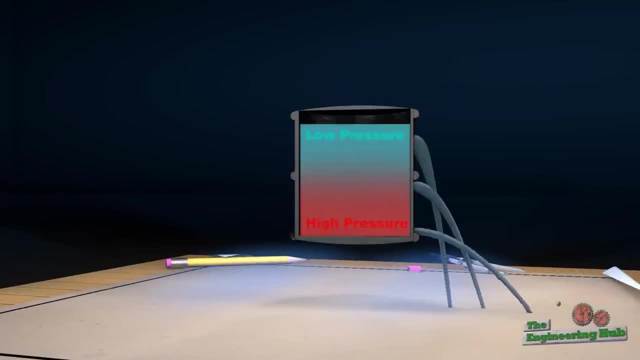 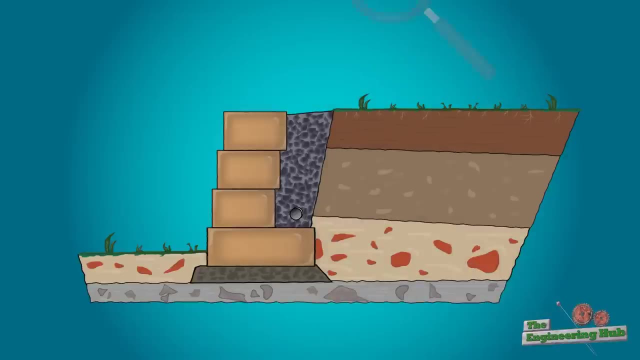 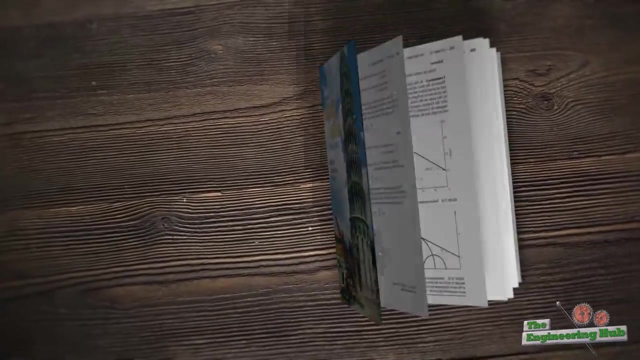 This pressure increases with the depth of soil. Unlike water, the pressure from the earth depends on whether the wall can move or not. In almost all practical cases, the wall does move and this helps relieve some of the pressure applied against it. Terzaghi, the father of soil mechanics, performed a bunch of full-scale tests on retaining walls. 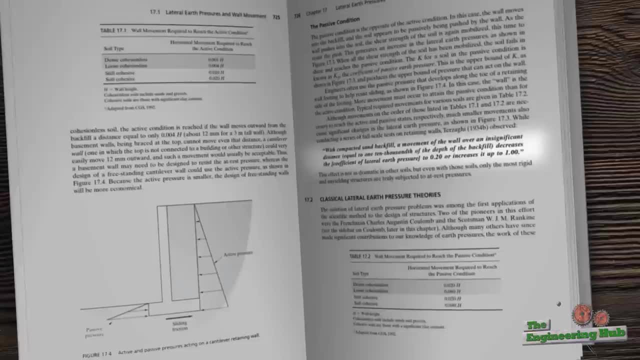 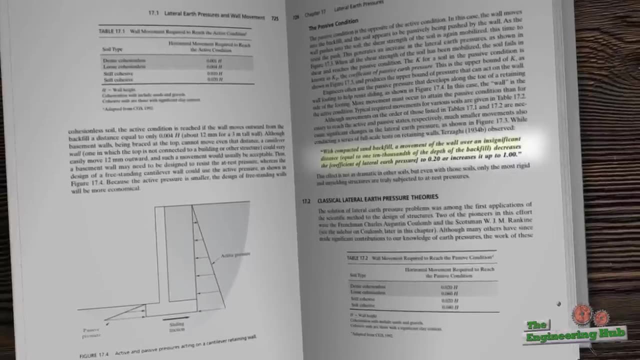 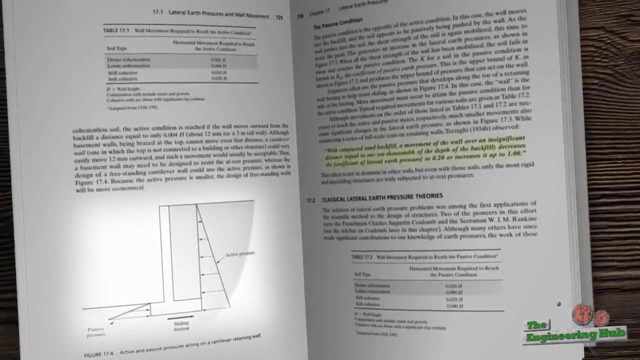 and found that even the most insignificant wall movements in the order of a fraction of a millimeter could reduce the lateral earth pressure applied to the wall by 50%. Theoretically, this reduction has to do with something called the active loading case and is related to the coefficient. 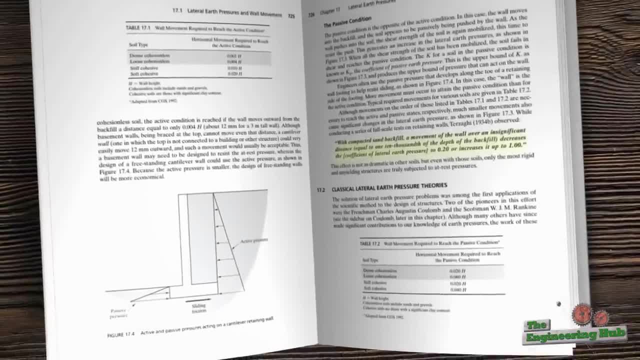 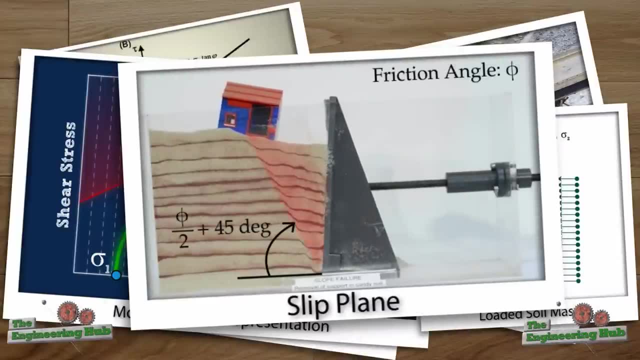 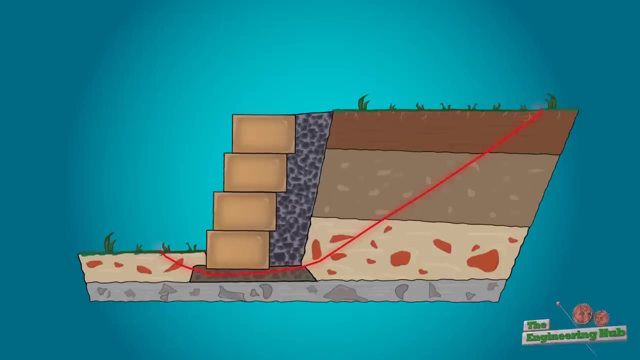 of lateral earth pressure. But instead of going into technicalities, we will try to explain this intuitively. When the wall moves, the soil wants to follow it and it starts to slide or separate from the main soil mass. We saw this in action in the previous video. This separation helps us. 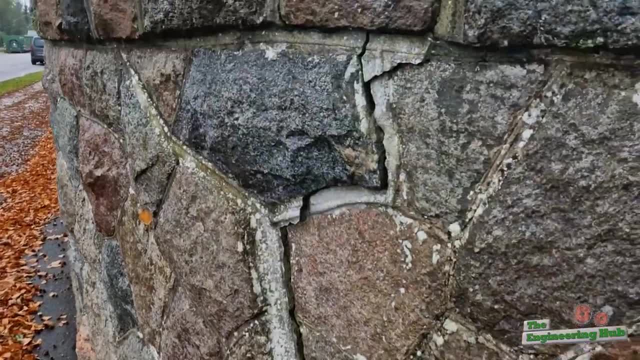 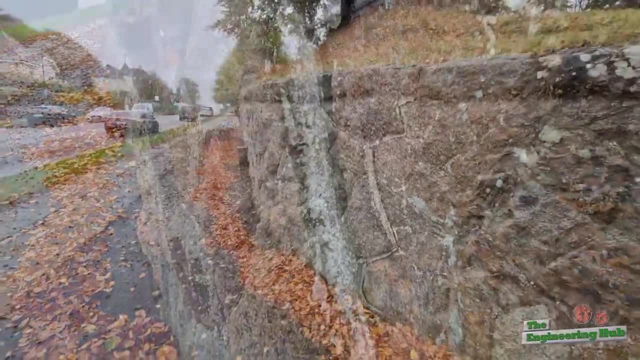 because the detached soil wedge has less mass and exerts a lower pressure than before the wall moved. Just to be clear, this movement is not visible by the naked eye. If you can visually see that the wall has moved, then you are probably looking at a failing wall. 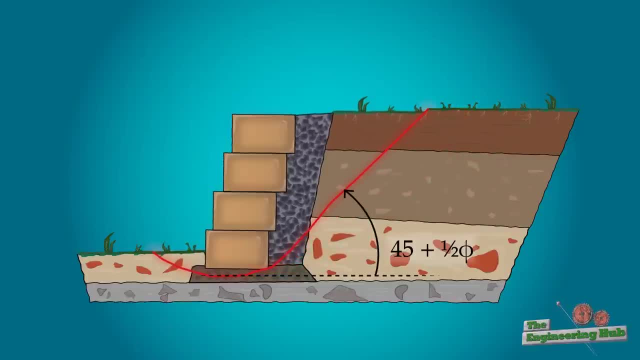 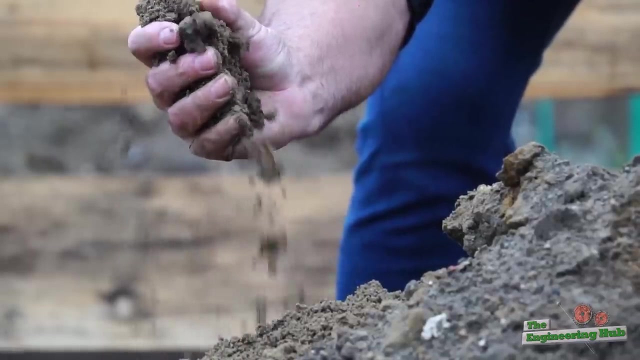 rather than the active loading case. So here you can see how increasing the friction angle of the soil decreases the pressure exerted on the wall. Now a good question is: how does one increase the friction angle? The friction angle is intrinsic to the type of soil, For example clays and silts. 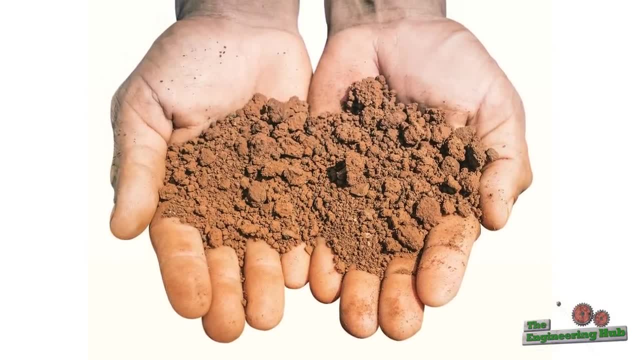 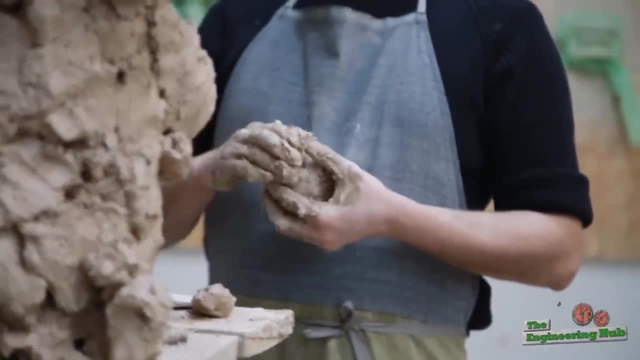 have low frictional strength. They use their cohesion or stickiness to carry the loads. The cohesive strength of the friction angle decreases the pressure exerted on the wall. The friction angle is unreliable because it could sometimes disappear if the soil gets saturated. Besides clays and 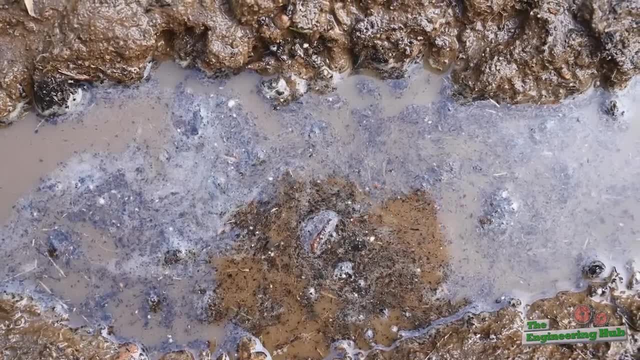 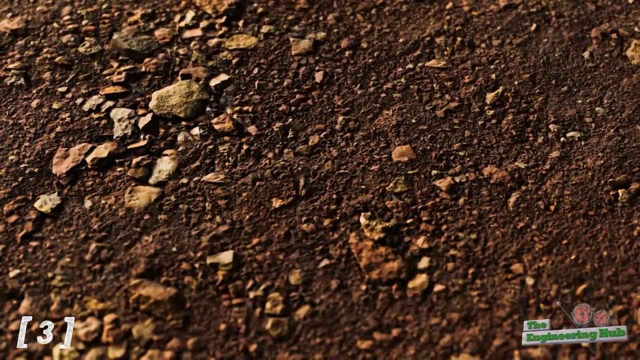 silts have low porosity and tend to trap the water, which is not something you want behind your wall. Granular soils like sands and gravels make for the best backfill material. They have decent friction angles and high hydraulic conductivity, which allows the water. 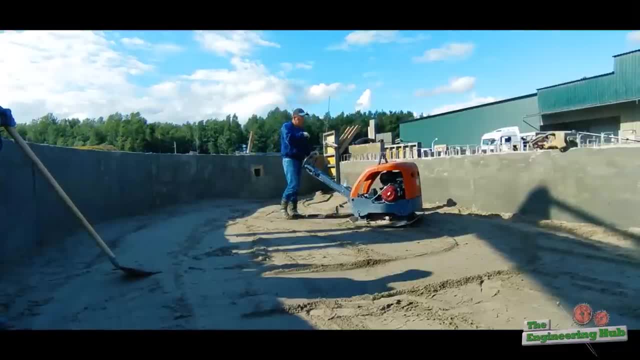 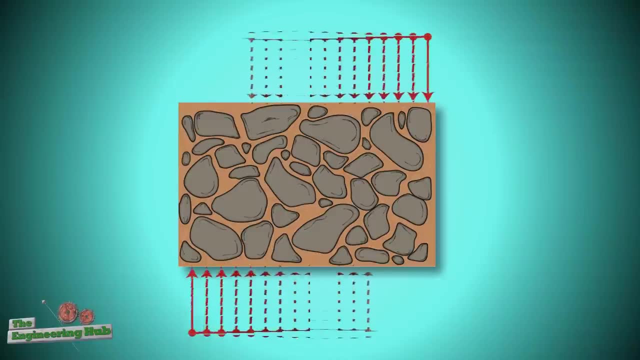 to easily drain, But to get the best out of your backfill, it is absolutely crucial to have the best part of the soil compacted. As we saw in the previous video, compacting the soils packs the particles tightly together, which significantly increases the friction angle and therefore, 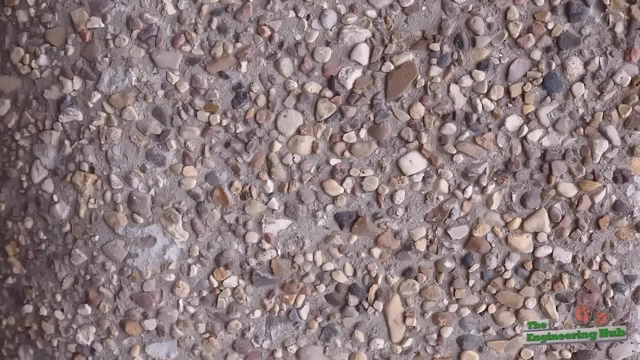 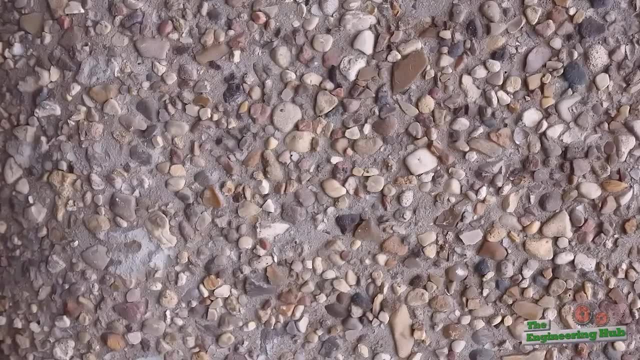 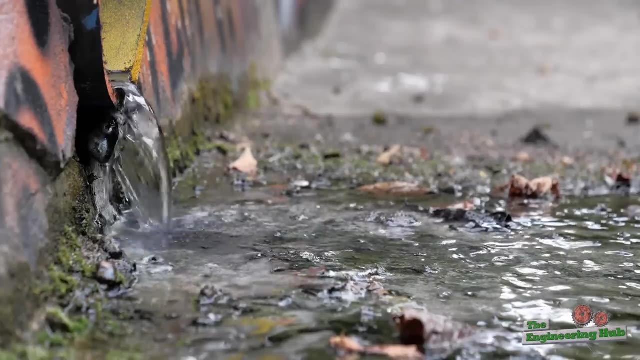 the strength of the soil. If the gravel is also well-graded, meaning the size of the particles is fairly uniformly distributed, then the strength is even better. The last point to make, before moving onto the actual wall scenarios, is about drainage. Providing drainage to the wall is 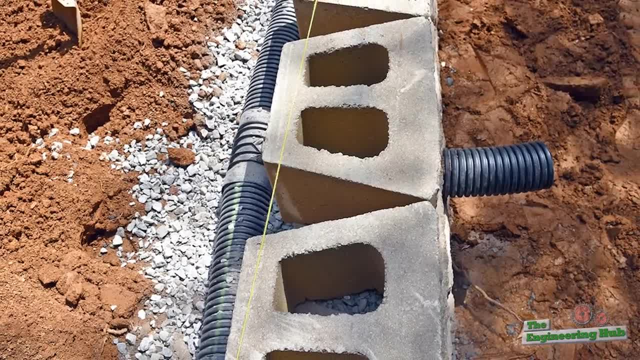 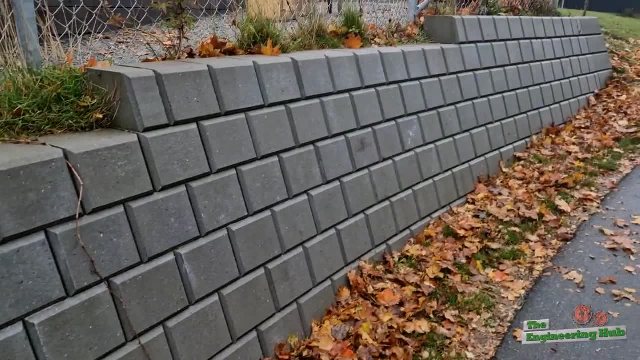 probably the most important thing, because the soil will be damaged if the soil is not well-graded. consideration, The effects of poor or no drainage will become apparent shortly Now let us look at a retaining wall design scenario and see how the soil parameters affect the factor of safety. If 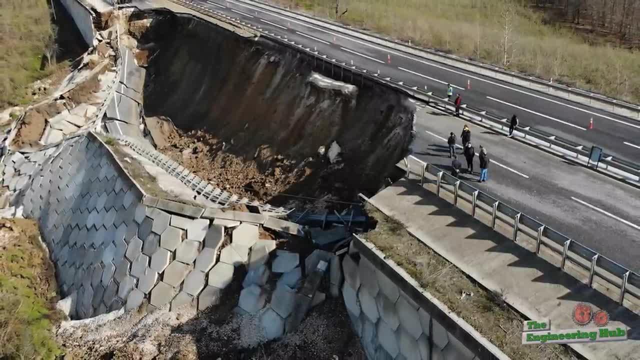 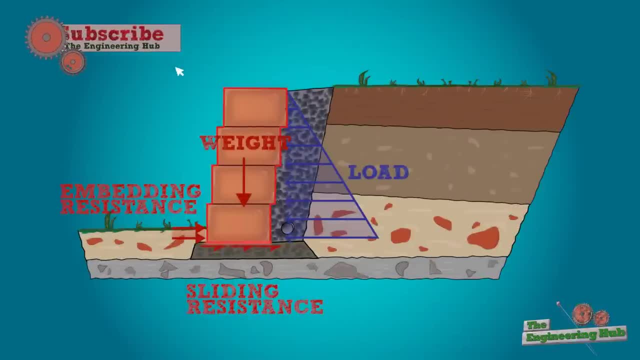 you are not familiar with the concept of a safety factor. it basically means how much the resistance of the wall is bigger than the driving force of the soil. A safety factor of 1 means that the two forces are equal and only a minor increase in the weight of the soil will cause a collapse.